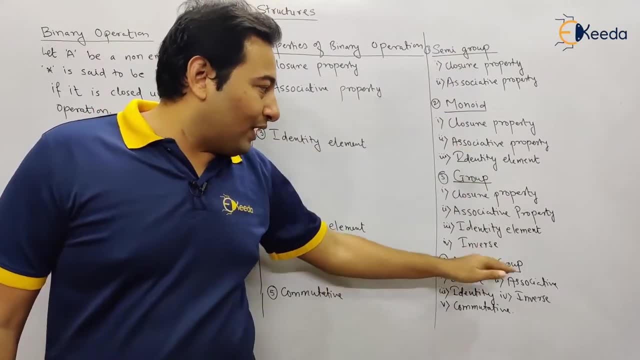 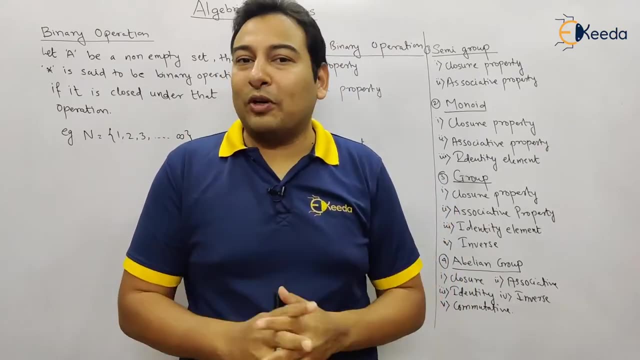 They are written here: semi group, monoid group, abelian group. There are few more: ring field, integral domain and so on. So these are the algebraic structure we are going to study under this particular chapter. So before going ahead, or before understanding what algebraic structure is, 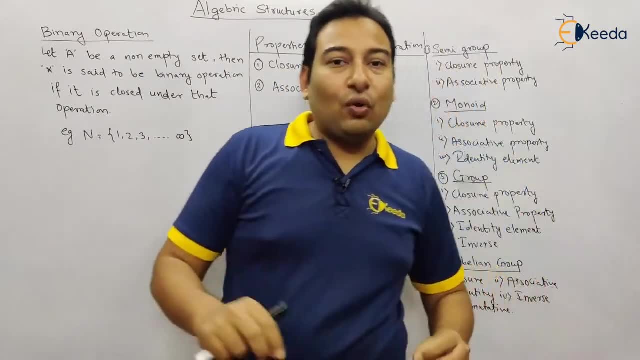 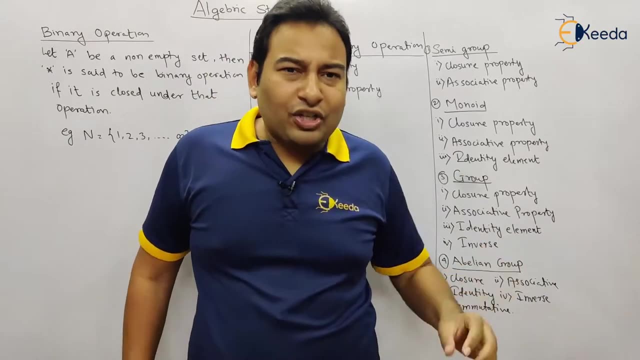 you need to understand what a binary operation is. So in this video we'll be discussing what binary operation is and what are the different properties. Because, see, once you are comfortable with the binary operation, you can easily manage and its properties obviously. Then you can easily 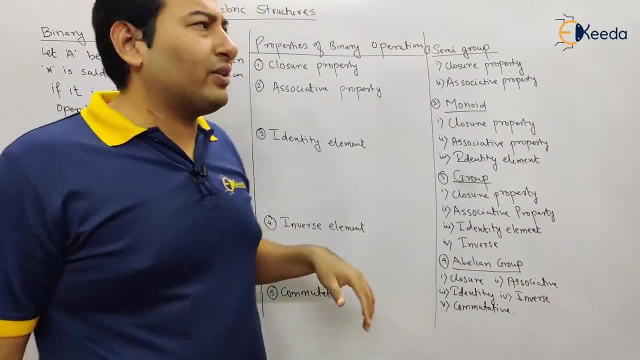 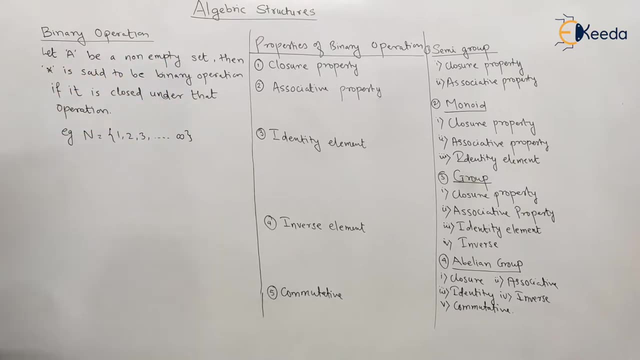 manage all the algebraic structure. So let us start. First of all, let us discuss the definition of algebraic structure. So let us start with the definition of algebraic structure. So let us start with the definition of a binary operation. Let A be a non-empty set, then star is set to be binary. 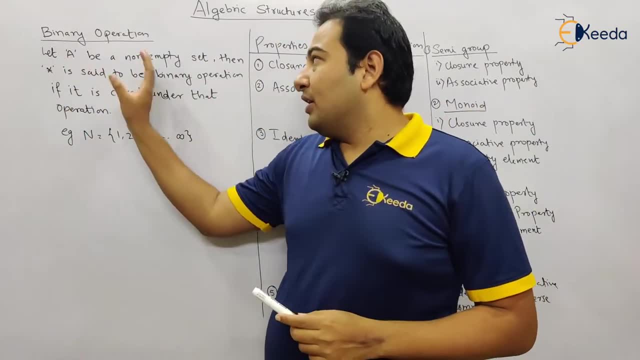 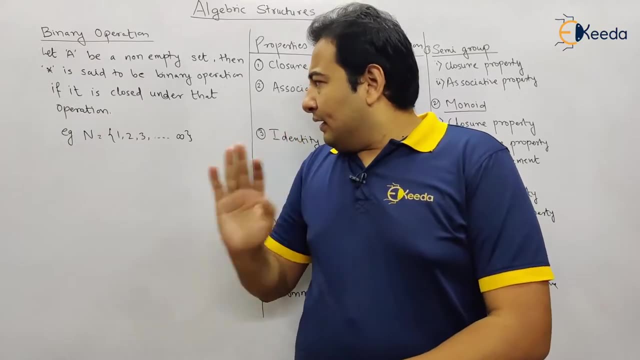 operation if it is closed under that operation. So this is the definition of binary operation. Now, what did you understand by this? Nothing, Don't worry, I'll explain you Now. there is an example given here. N is equal to set of natural numbers If you add any two. 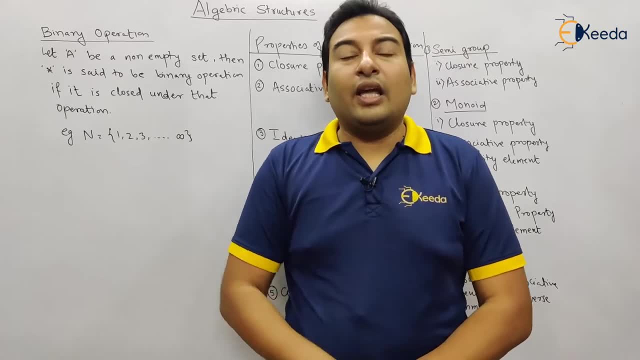 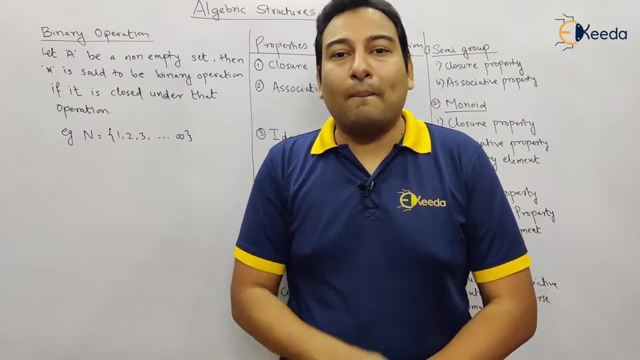 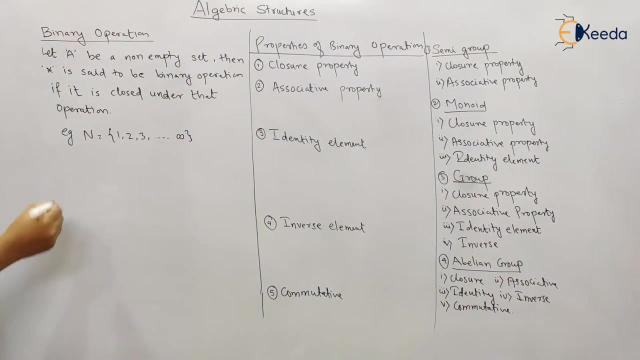 natural numbers. Let's say 2 and 3. If you add any two natural numbers, your result will be also be a natural number. Agree, Therefore N plus is closed, or it's simply called. it's a binary operation. So are you clear with the definition? See, N plus is a binary operation. Now what is? 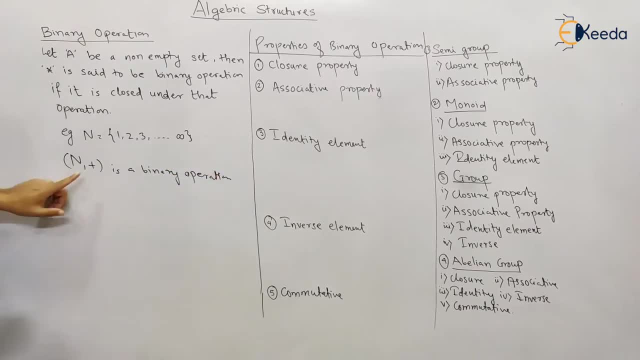 the definition. If you perform this particular operation, Here it is star. Star means a general operation, But here we are taking a specific operation- If you are performing addition on this particular operation. So if you perform addition on this particular operation, So if you 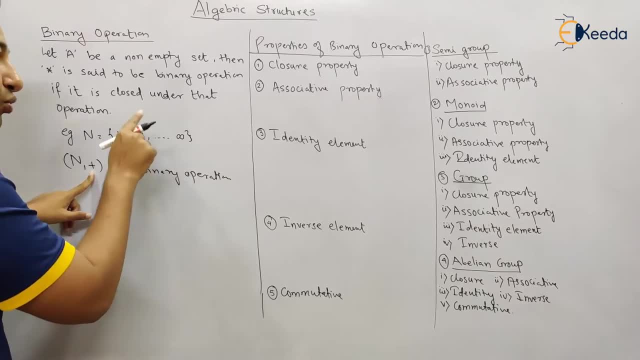 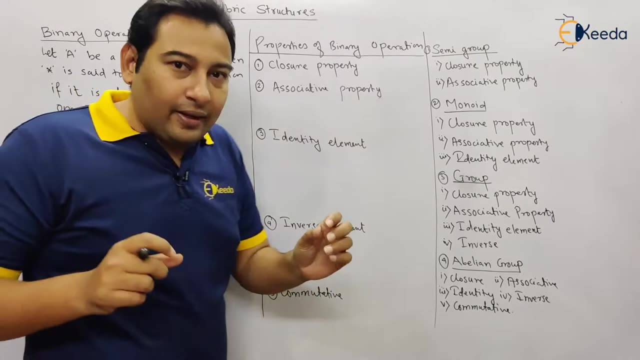 perform this particular set- natural numbers, So any two numbers. if you're taking addition, your result will also be a natural number. Therefore it is called closed. Closed means perform the operation on the set and the result should also belong to the set. If this is the condition, 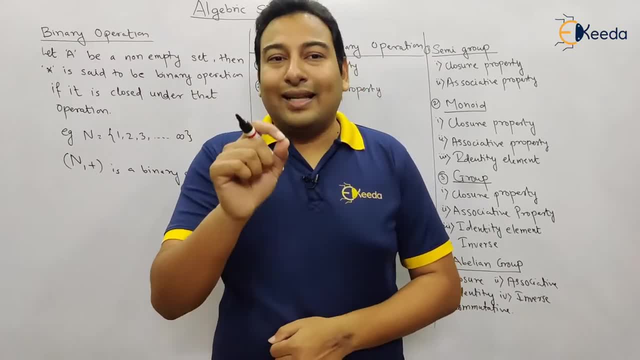 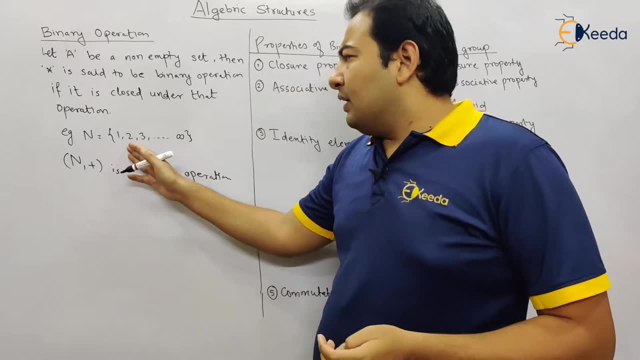 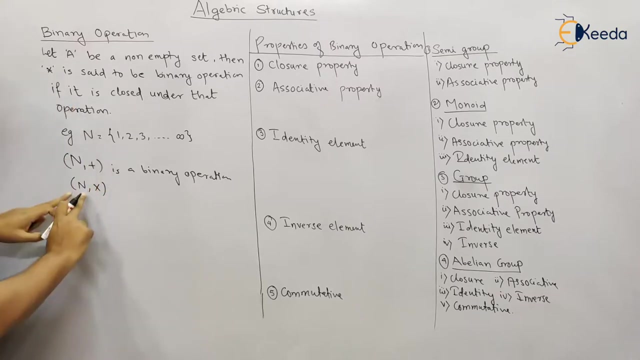 satisfied, then it is called closed and in that case that set comma operation becomes the binary operation. Are you clear with this? Let me give you one more example. Let's say N comma star or N comma multiplication- basically I'm not using star because star is a general operation- N comma- 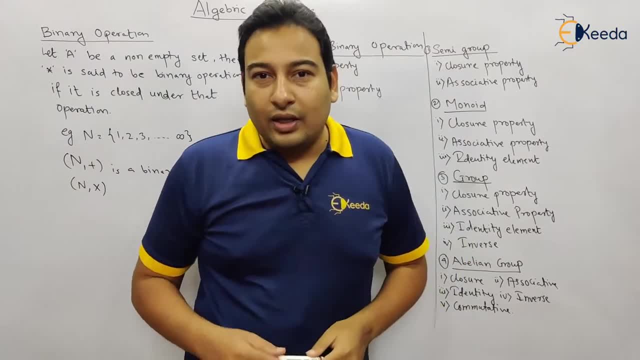 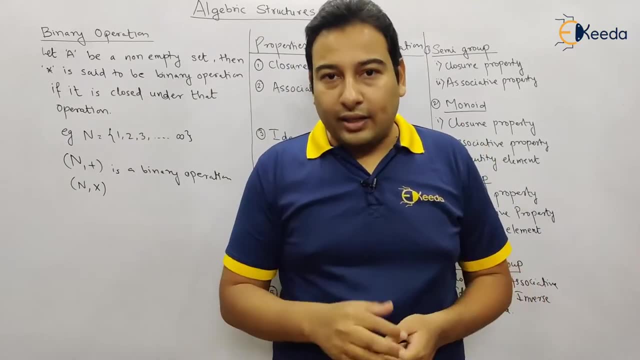 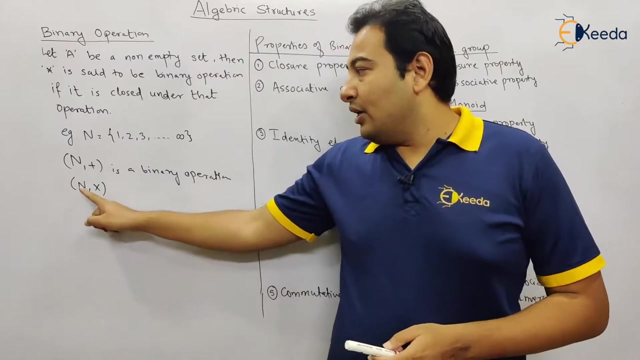 into? Please tell me, is it a binary operation? So what is the condition? Consider any two elements from this set natural number and multiply. Let's say 2 and 3.. So if you multiply 2 and 3, the result is 6.. That also is a natural number. Therefore you can say N comma. multiplication is closed. 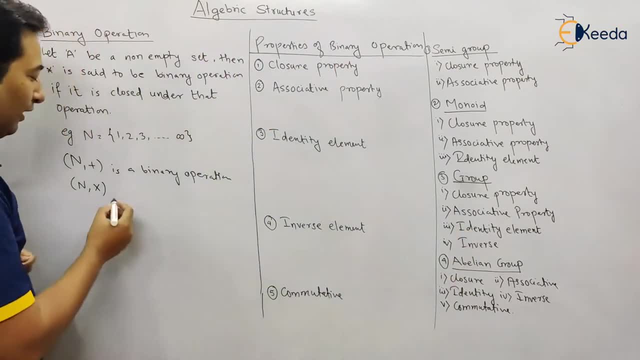 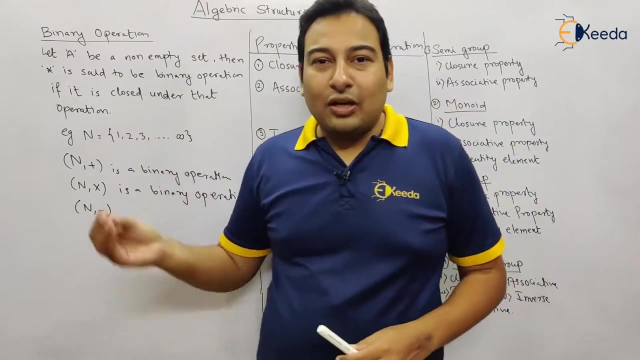 operation and therefore it is called a binary operation. Therefore, N comma multiplication is also a binary operation. Now let me give you an example which is not a binary operation. Now please tell me: N comma minus, Is it a binary operation or not? No, Take any two natural. 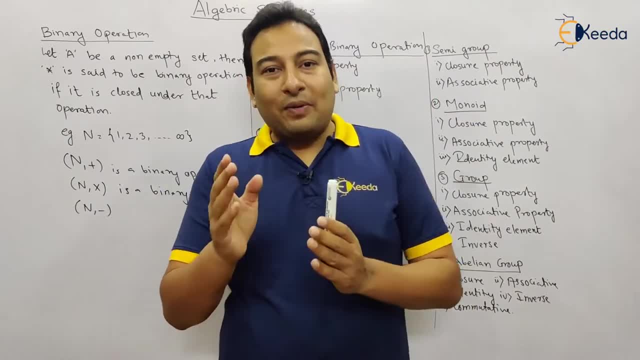 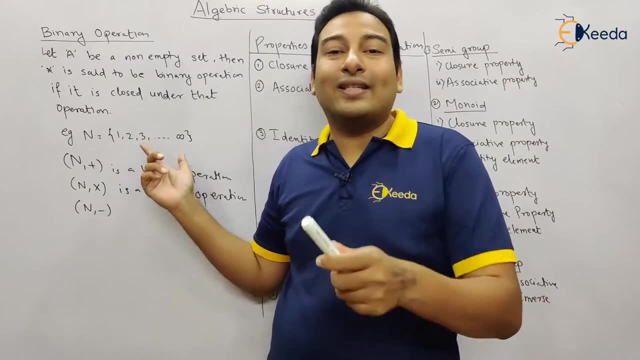 numbers. Let's say 2 and 3.. So if you subtract 3 minus 2, that is okay, because 3 minus 2 is what 1 that belongs to the set. But what if you do 2 minus 3? So 2 minus 3 is what Minus 1 and minus. 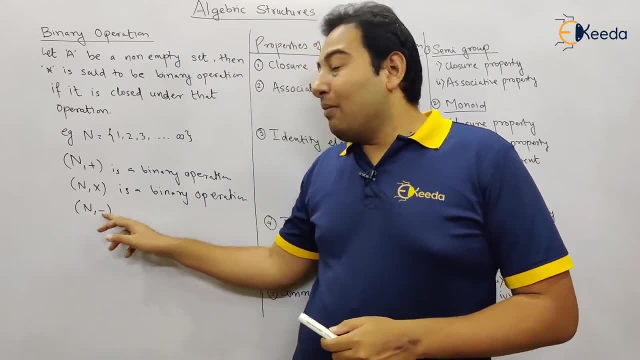 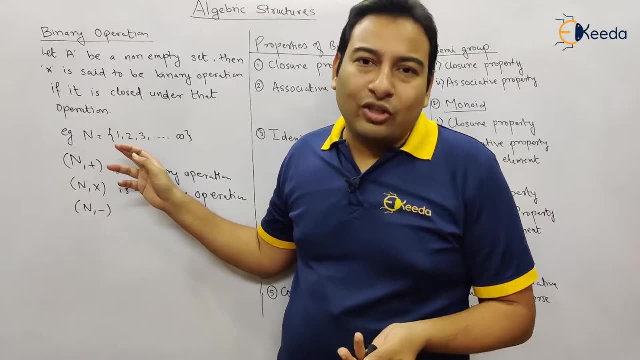 1 does not belong to this particular set. Therefore N comma minus is not closed. Therefore it's not a binary operation. or simply you can say: take same number, Let's say 2 minus 2.. So 2 minus 2 is what, 0.. 0 again does not belong to the. 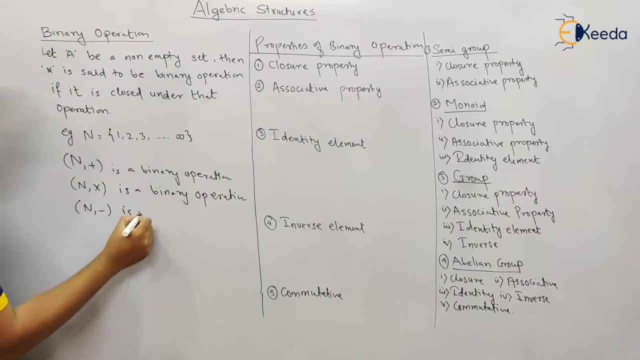 natural number. Therefore it is not a binary operation. Is this definition clear of binary operation? So what is the definition of binary operation? A be a non-empty set, Likewise here it is N. Star is said to be binary operation, Likewise plus or multiplication. 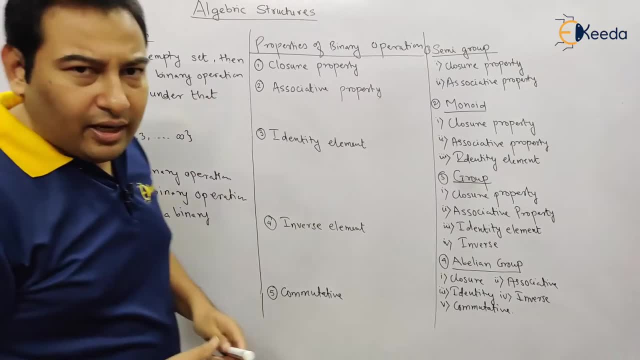 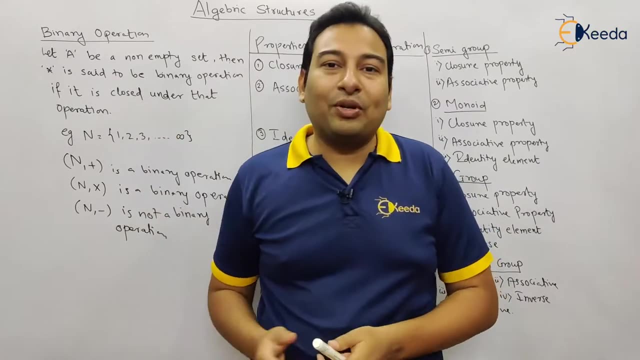 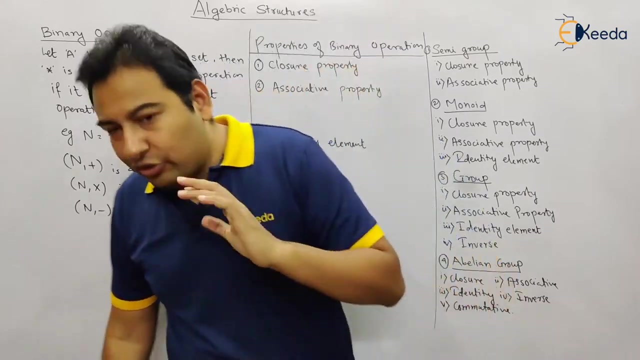 If it is closed under that operation. that means: take any two numbers, perform that operation. If result is also present in that set, then it is called a binary operation. If it is not present, then it is not a binary operation. Is this definition clear of binary operation? Yes, Let's. 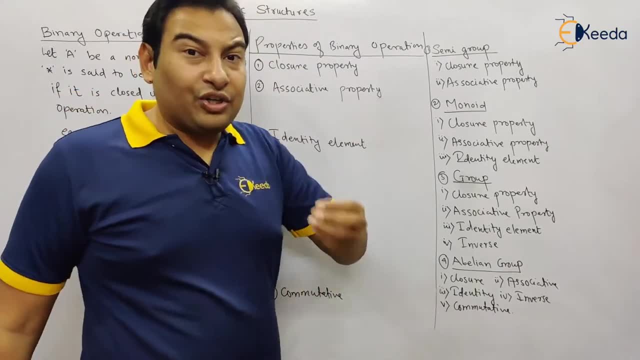 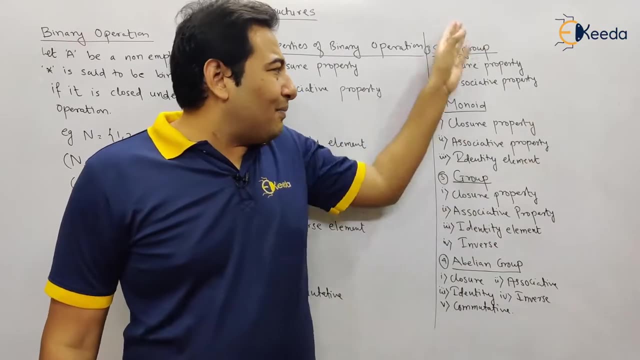 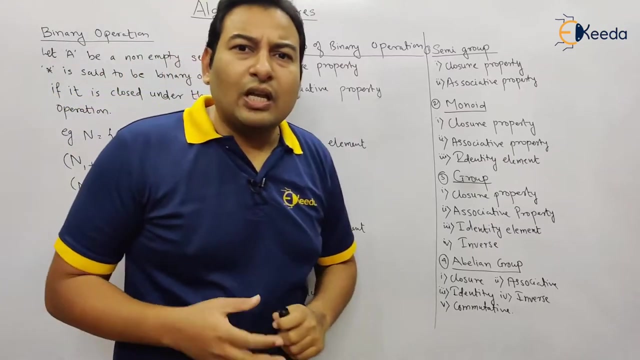 move on. Now we'll discuss what are the different properties of binary operation. Very important, Very important lecture. You need to understand these properties because if you understood these properties, you can easily manage all the algebraic structure. So let us start. The first property is closure property. Closure property means the same thing. 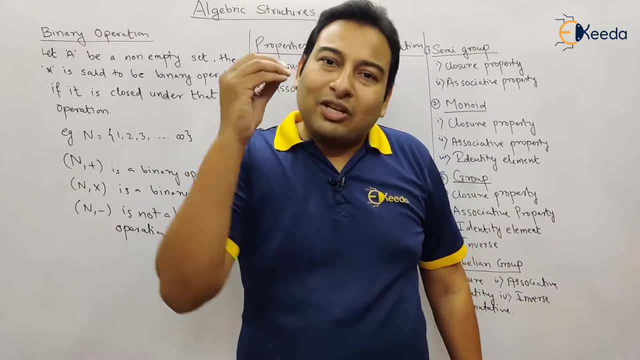 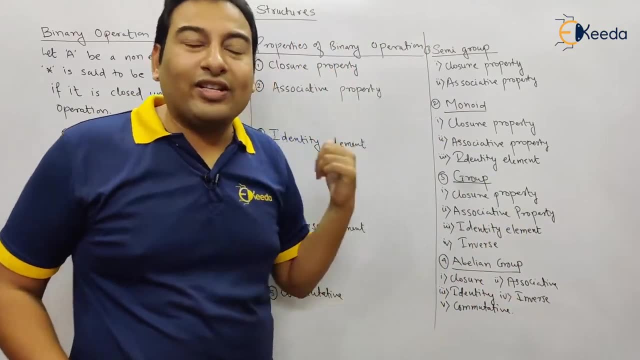 that we just discussed, An operation must be closed, or simply, if it is closed, then only it is called binary operation. So that is the first property that we already discussed. And what is the closure property? Take any two numbers, perform that operation. The result should also present in. 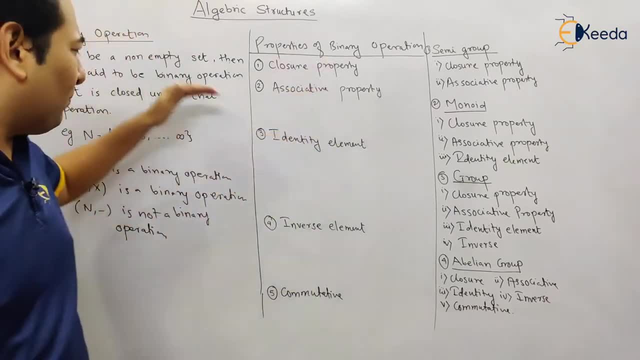 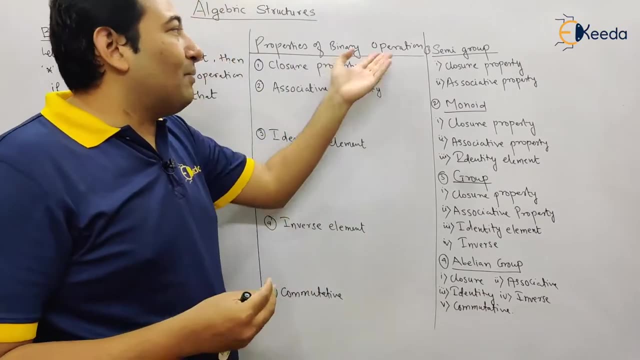 that set, Then it is called a closed operation or it is called closure property, The same thing that we discussed. So obviously closure property is a closed operation. So if it is closed, then only the property must be satisfied. If it is not satisfied, then it is not a binary operation. So 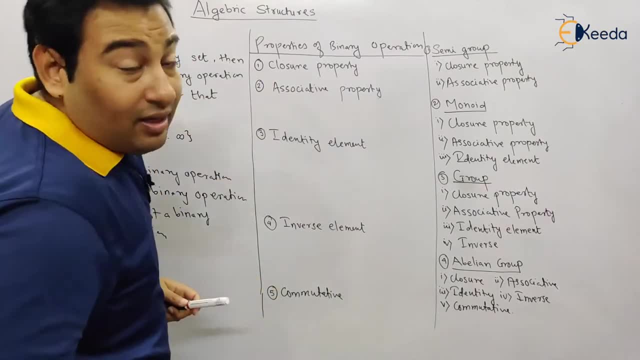 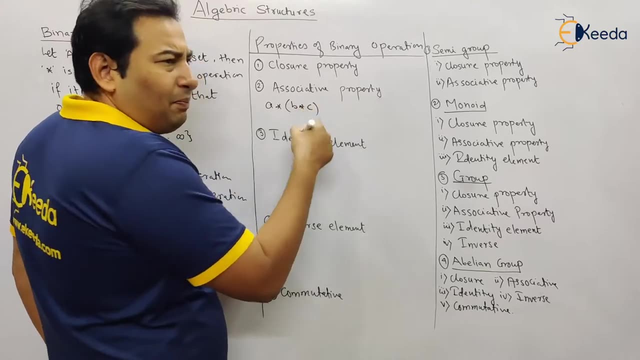 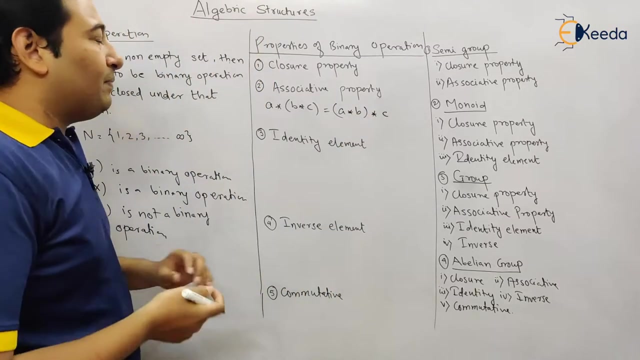 first property is closure property. What is the next property? Property number two is associative property. So what is the associative property? Let's say, star is any operation. It can be plus, minus, addition, multiplication, whatever. So this property is called your associative property. That. 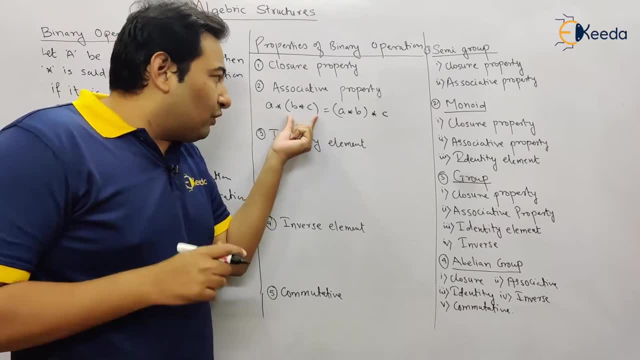 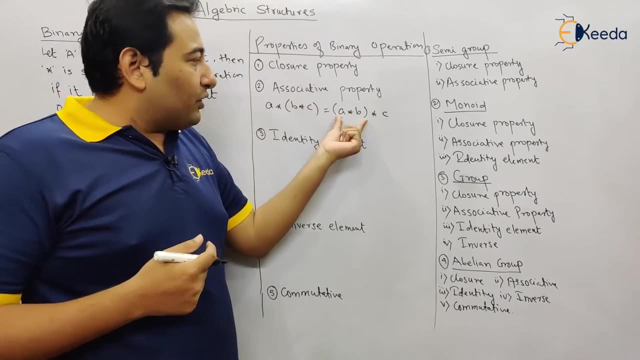 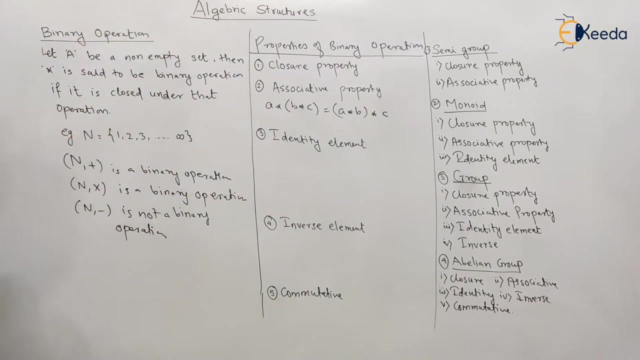 means, if this is your expression, first of all this particular bracket will be evaluated and after that, result of this, And here, first of all, this will be evaluated, and with the result of this bracket, star c. So obviously you know this associative property. Next, identity element: very 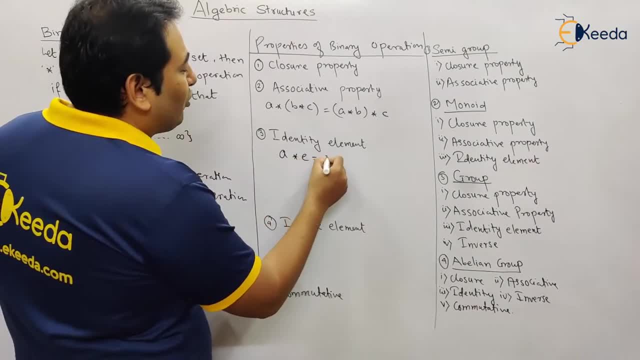 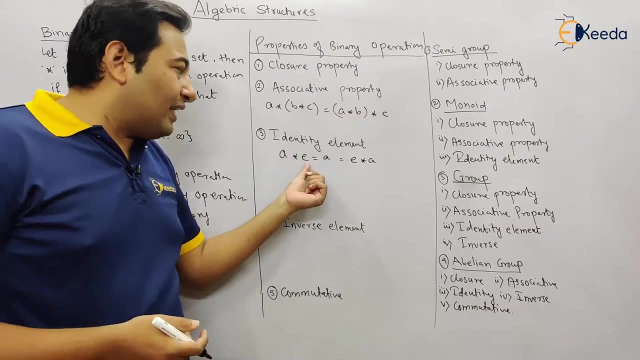 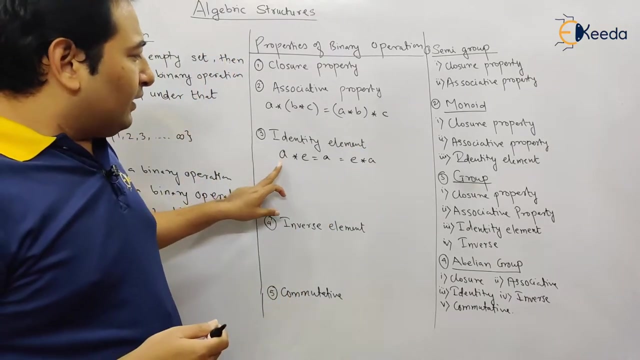 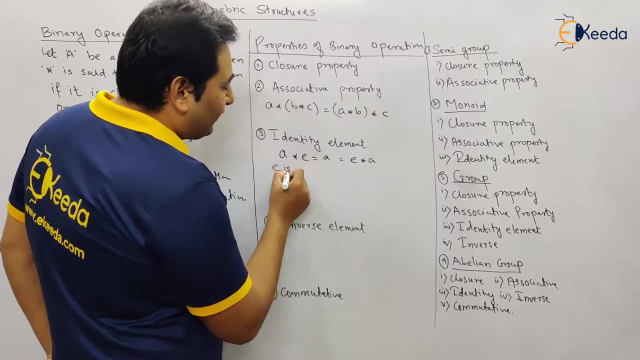 important property and the property says a star e is equal to a, or simply say e star a. In short, a star e or e star a- doesn't matter, Just concentrate here on this particular term so that this will be very clear- Also mean the same: a star e is equal to a. If this is the case, e is identity element. If this: 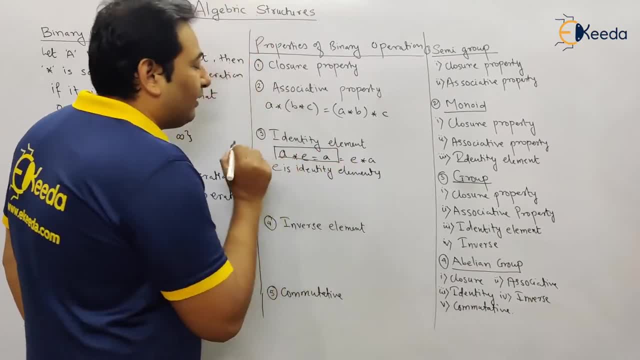 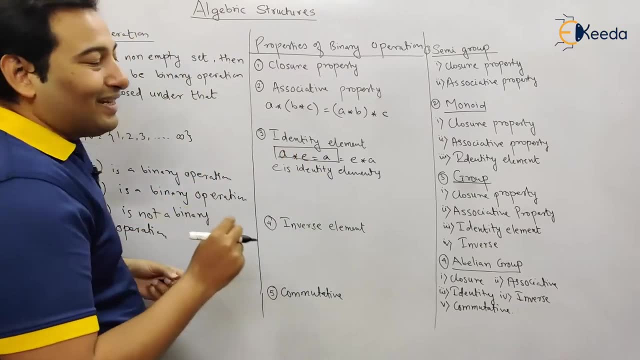 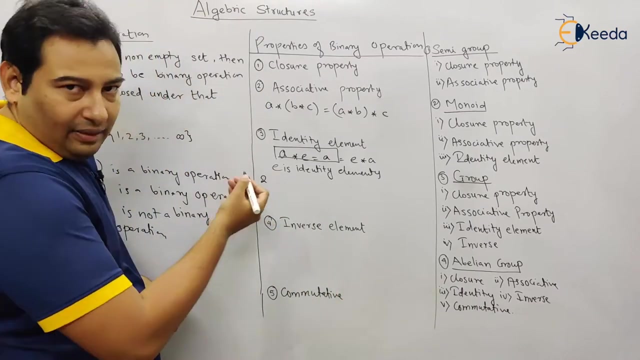 definition is satisfied, then e is your identity element. So this is the definition. So what is the definition? See, you should get the same term. You should get the same term. Now let us identify what is the identity element with respect to plus. See here two. Let me take two as an element. 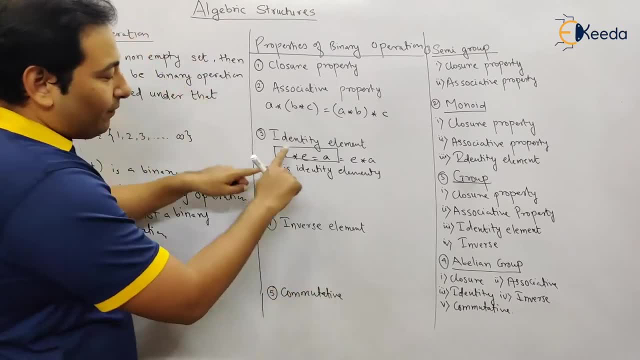 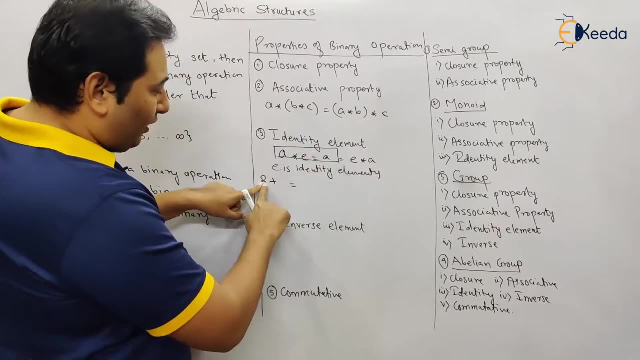 Let me take the operation plus. And what is the definition says: Whatever you write here, you should write here. Whatever you write here, you should write here. We should get the same answer. So here we have two, So we should get two. 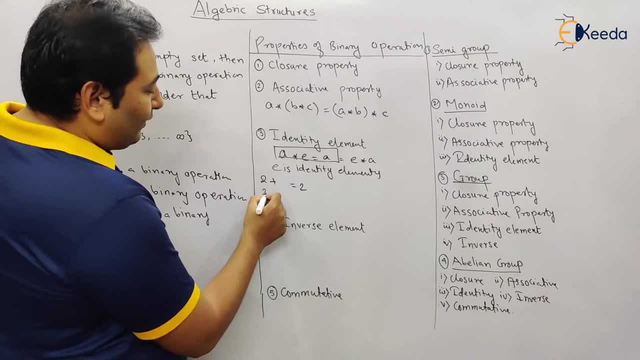 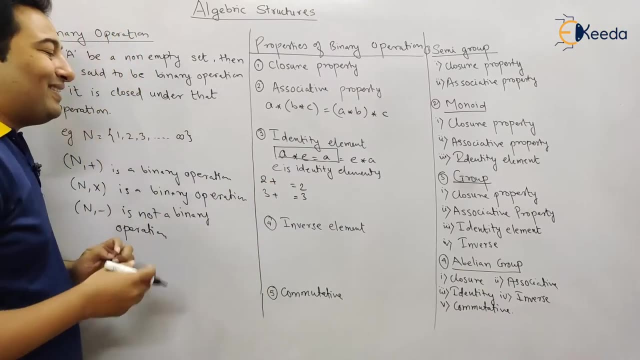 Let me take one more example. Let's say three. So whatever we write here, See here a and a. So whatever comes here is your identity element. Now please tell me, what should I write here so that I will get? the answer is two and the answer is zero. 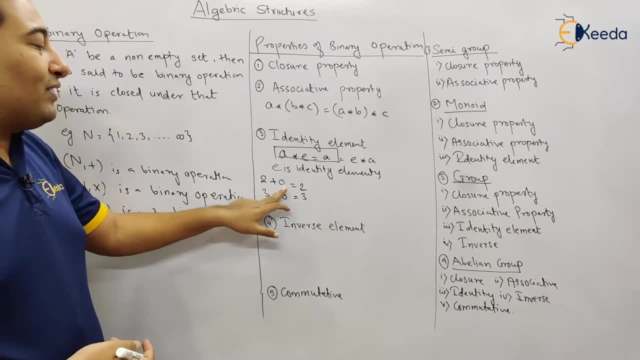 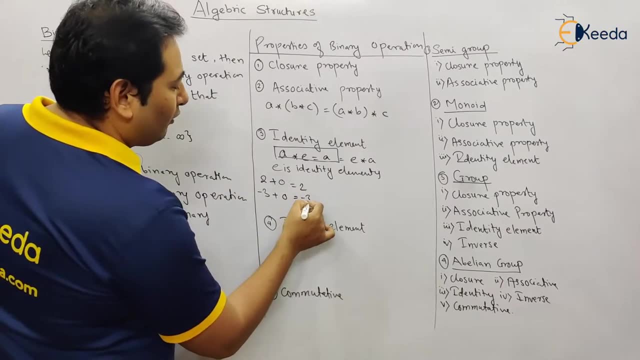 So if I'll write zero here, So this is two plus zero equal to two, Three plus zero equal to three, Or in fact you can take negative number also, So see here. So in short, e is equal to zero. So what is the identity element with respect to plus? 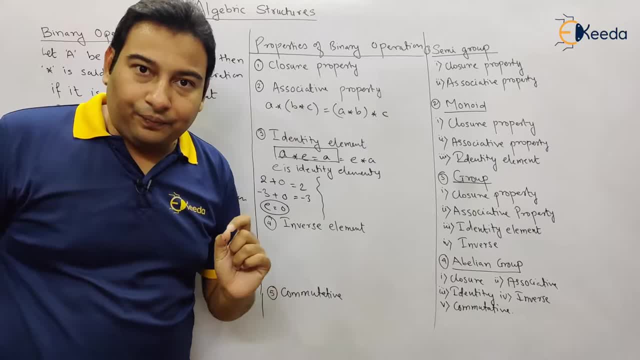 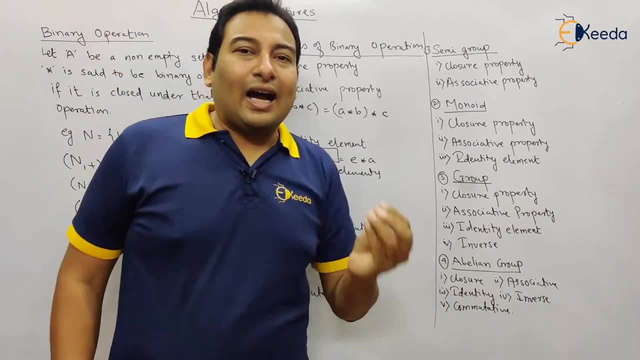 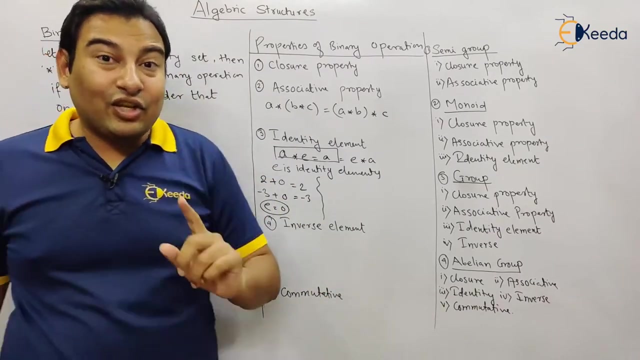 Identity element with respect to plus is zero. Generally what we say identity element is one, But forget about the normal mathematics. We are into discrete mathematics. Generally, what we say identity element is one, But not here. Here e is equal to zero. Identity element is zero. 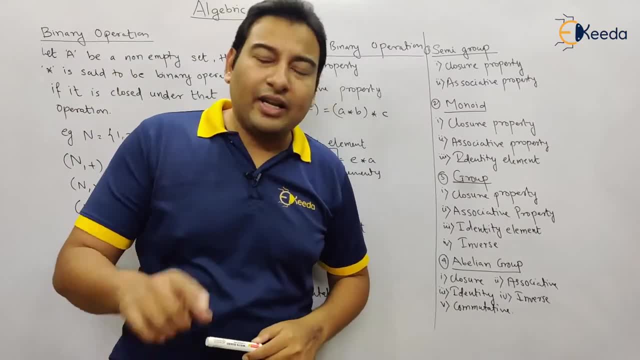 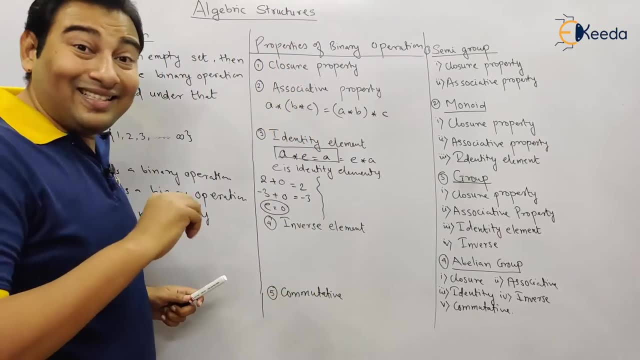 So whenever I ask you what is the identity element, you should ask me first, Sir, with respect to which operation? So with respect to plus e is your identity element? That is, e is zero is your identity element. Now let us talk identity element with respect to multiplication. 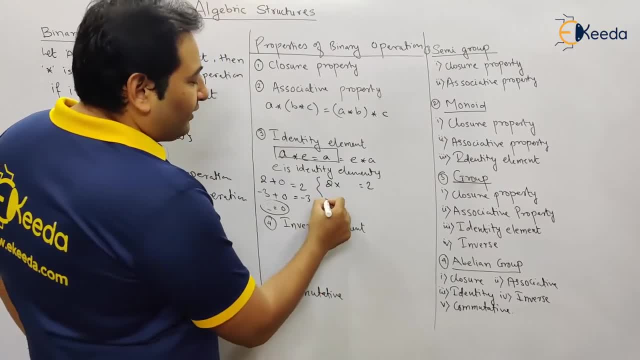 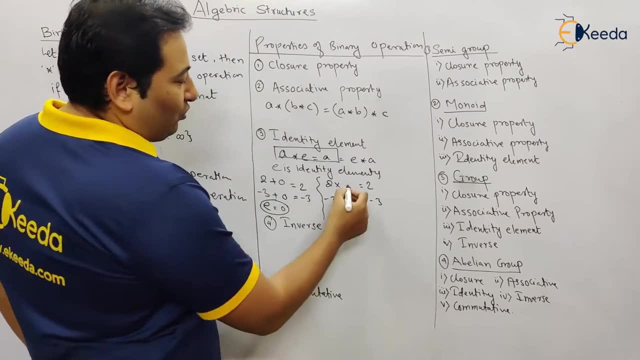 So here two, You should get two. Let's say minus three, So you should get minus three. Now, what should I write here? I should write one. If I write one, see here: Two into one is two, Minus three into one is minus three. In short, e is equal to one. 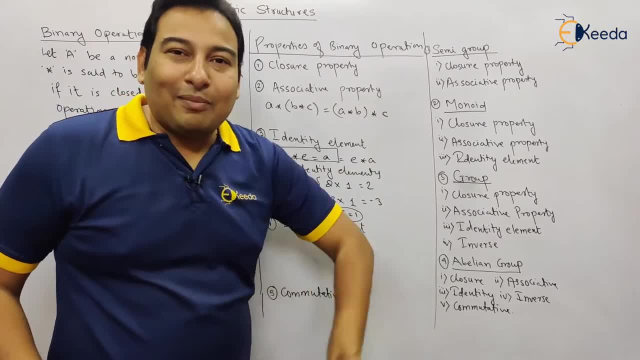 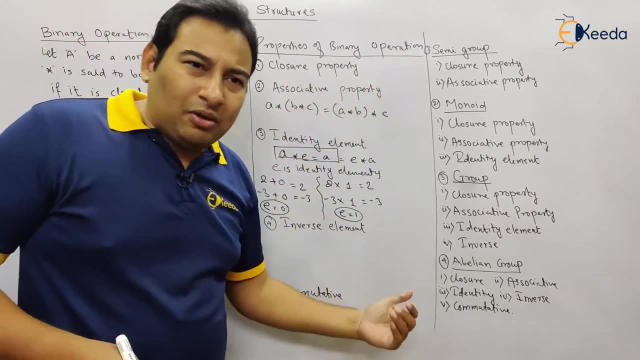 That means, with respect to multiplication, my identity element is one. Is this clear? how to find it out, the identity element? And don't worry, While solving the problem, we're going to consider these things in detail. So you just need to understand the concept first, Because here and there, few variation. 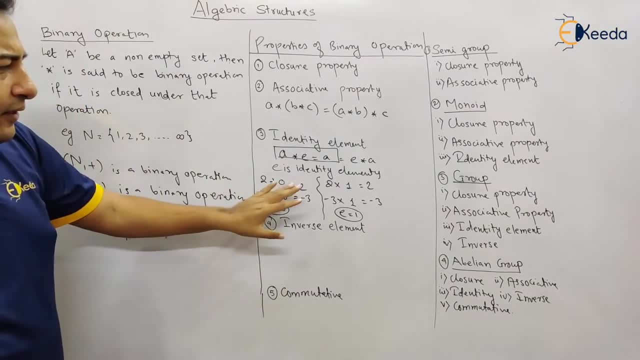 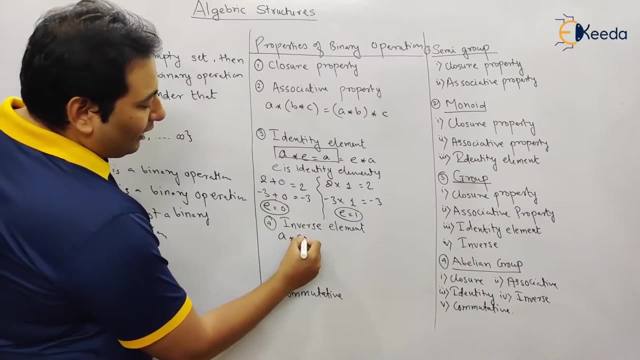 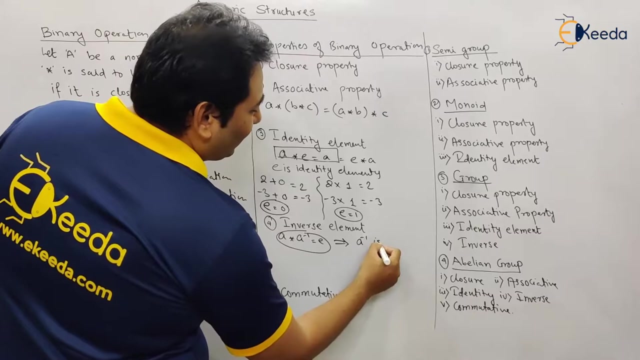 and you will be able to manage the algebraic structures. So this is the concept of identity. Next, let's talk about the inverse Now. inverse means a star. a inverse is equal to e. If this is the case, a inverse is your, basically inverse. 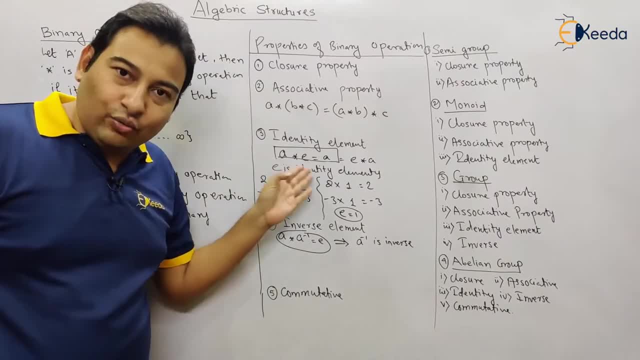 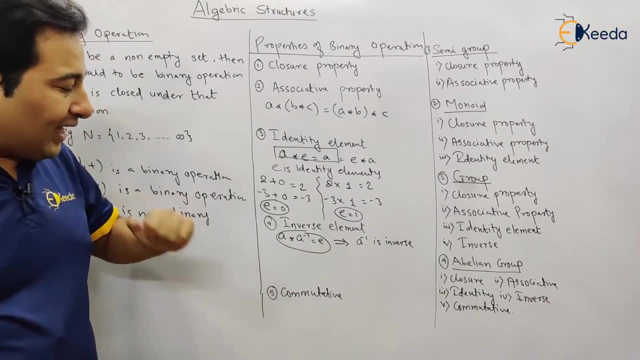 Now, this is the definition that you need to remember. Likewise, identity: you need to remember the definition. Here also, you need to remember the definition And what the definition says. a star, a inverse equal to e. That means here it should be a and here should be a. 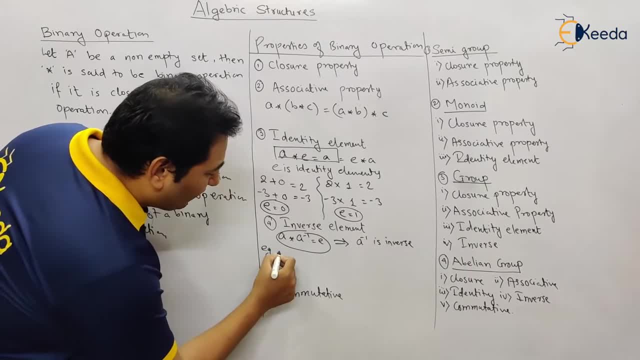 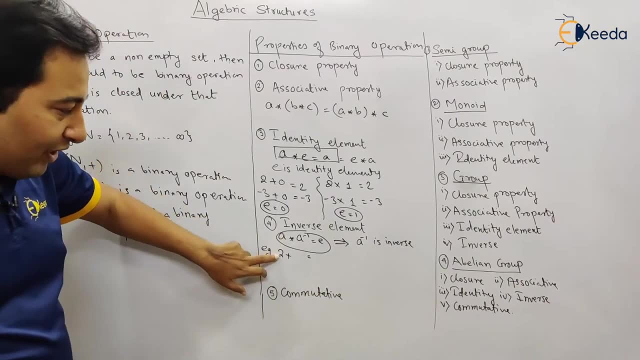 let me take examples So that it will be clear. Let me take two, And if I say I take plus here, I should get the identity element In place of a. I'm taking two in place of a star. I'm taking plus Here. I should get, on right hand side, my identity element. 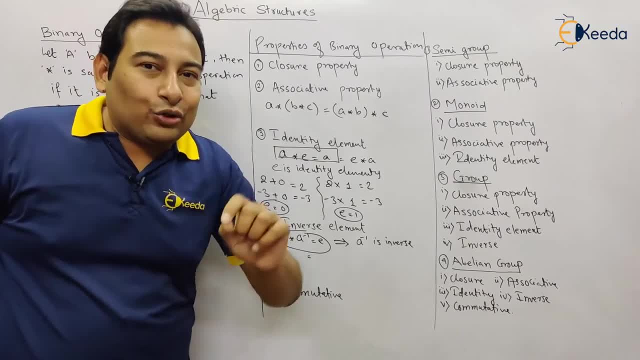 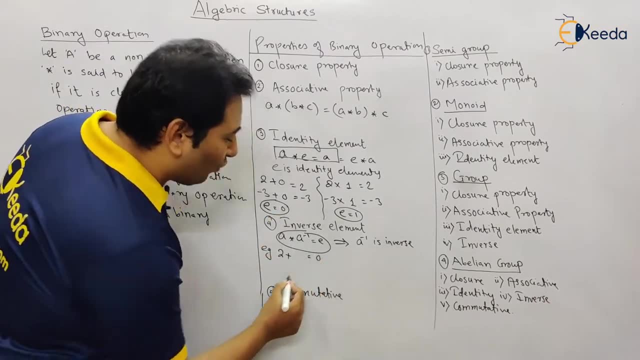 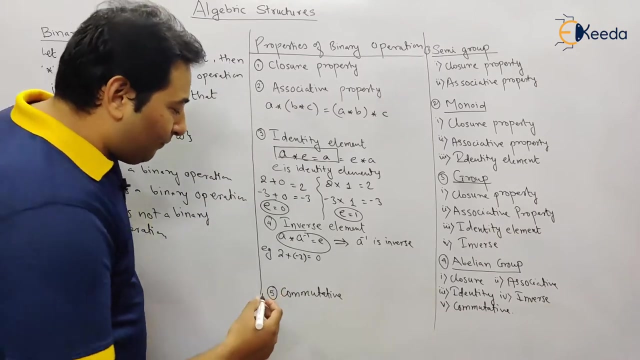 Now, what is the operation? what is identity element? first of all, Yes, valid question. with respect to which operation? here we are talking about plus, so what it should be the identity element? should it be zero? So write here two or two as an example to get zero. so i should write minus two. that means two inverse is minus two, that means a inverse is. 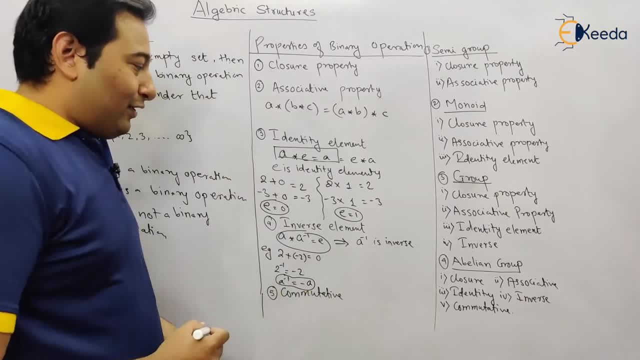 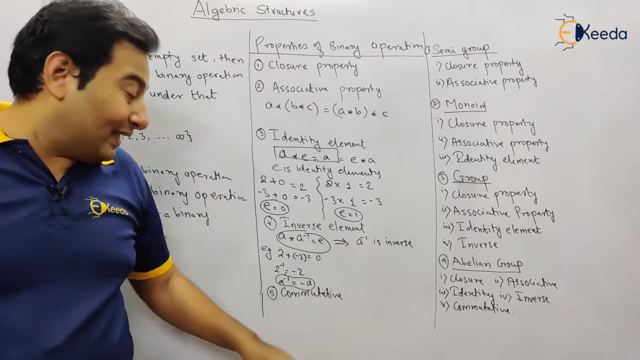 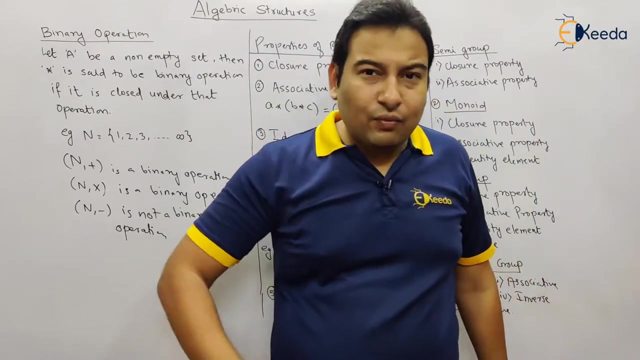 minus a. is this clear? generally, what we say a inverse, a inverse is one upon a, but this is not the case here. a inverse is minus a, so it's not a general mathematics. so whenever i ask you, what is the identity element, what is the inverse, the first question should come in your mind is: 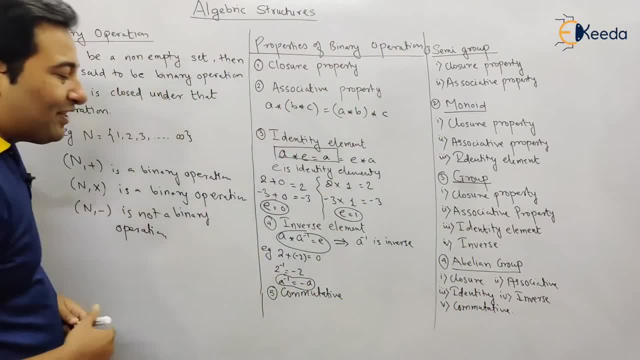 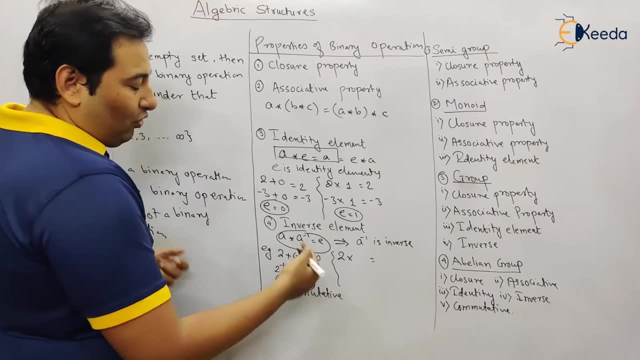 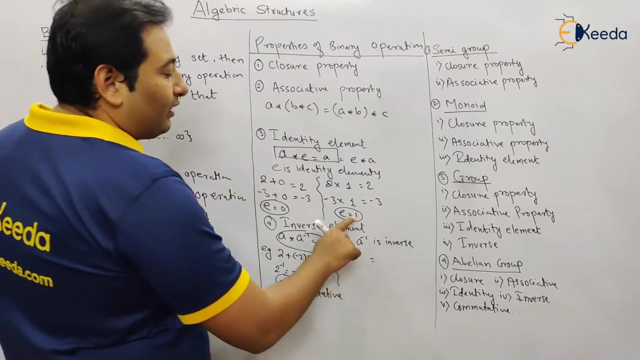 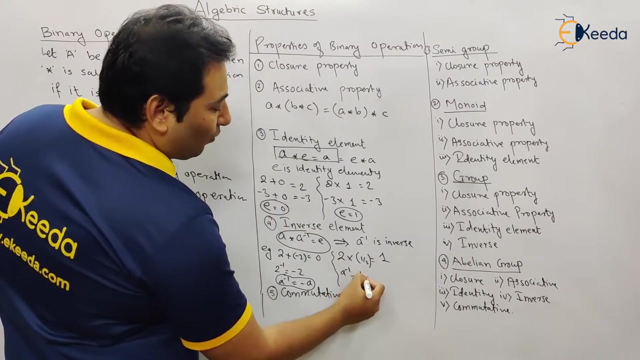 so with respect to which operation? now let us discuss the same example with respect to multiplication. here it is two star multiplication, not star. basically, e is the identity element. now we are talking about multiplication. so what is the identity element? now, it should be one here. so what should i write? here is one upon two, so you can say: a inverse is one upon a. 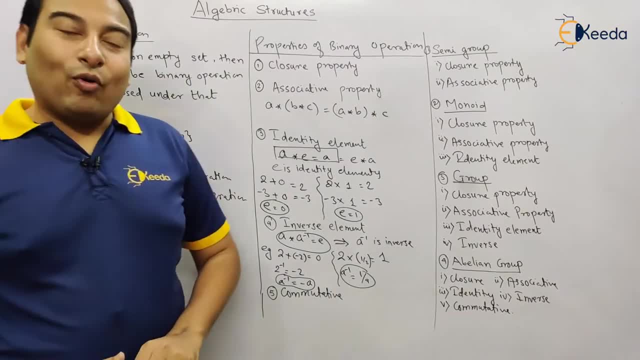 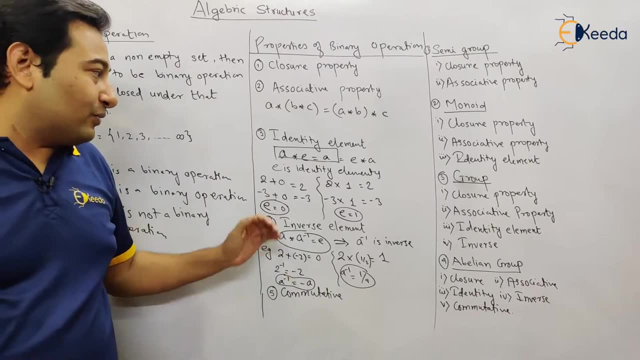 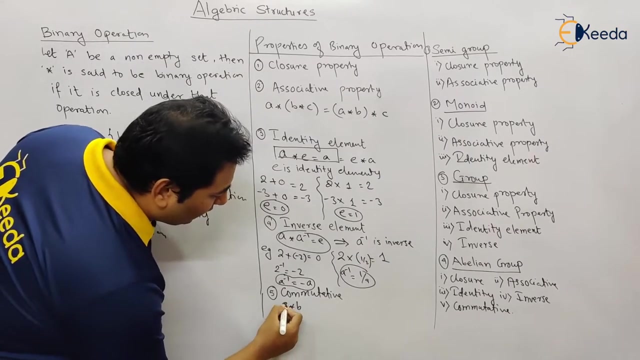 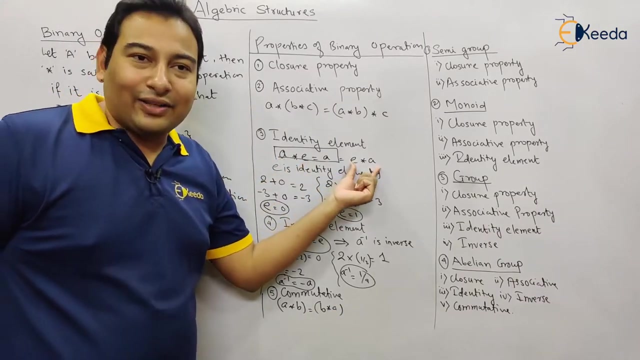 a inverse is one upon a with respect what, with respect to multiplication, but a inverse is minus a with respect to addition. so you should know these things. so i think this is clear: identity element and inverse. let's discuss commutative. it's very simple. property: a star b is equal to b star a, see here. a star e is star a. so 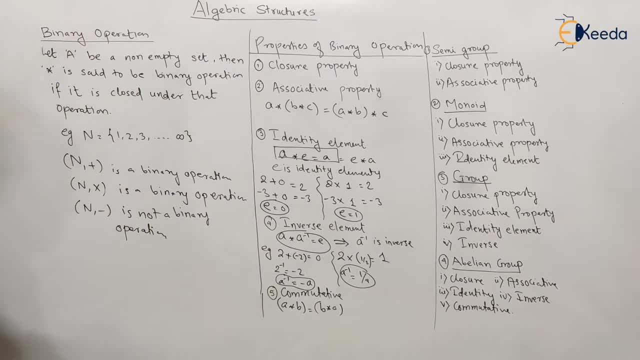 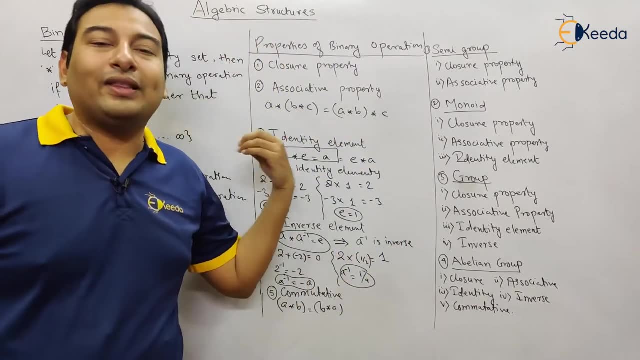 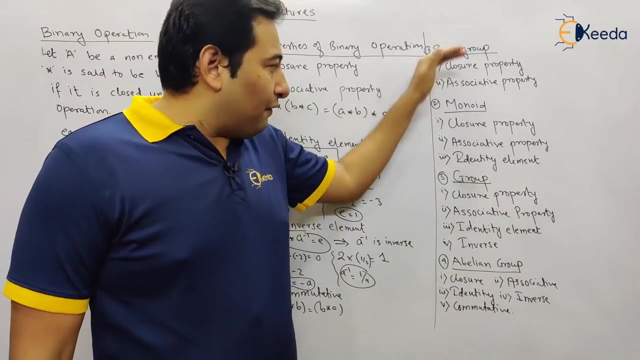 that is your commutative property. a star b is equal to b star a. so these are the different properties of binary operation. so i hope these properties are clear, along with the definition of binary operation. now let us discuss what are the different algebraic structure. so there are. 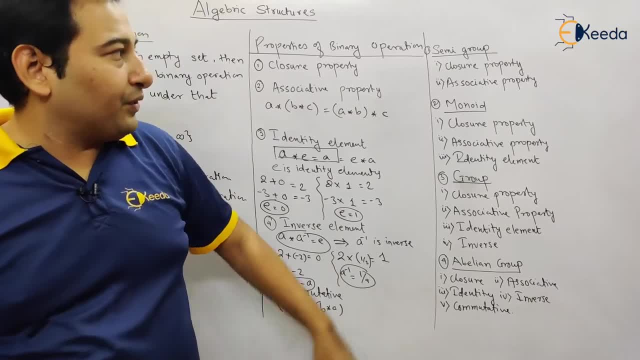 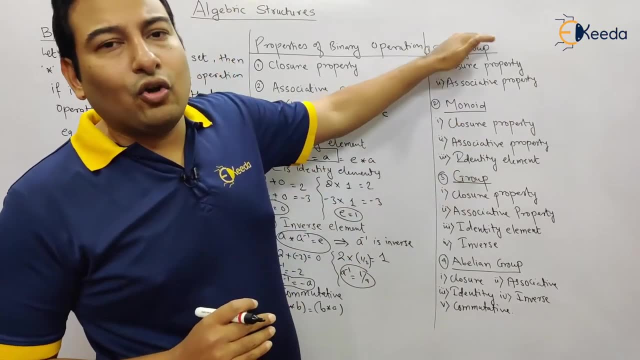 four algebraic structure that we are going to discuss here in the next videos, coming videos, and there are few more also, but yes, we divide into two parts. basically you can say, in the first discussion we'll talk about these four algebraic structure. the first algebraic structure is semi.